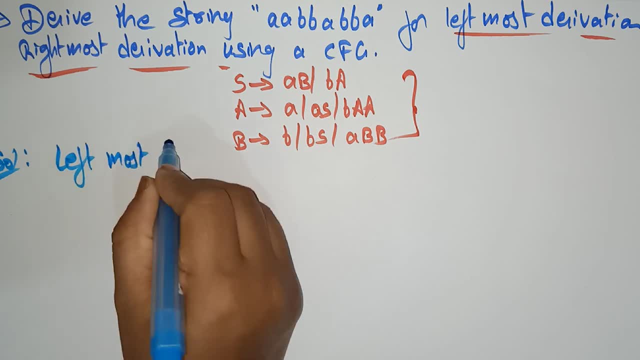 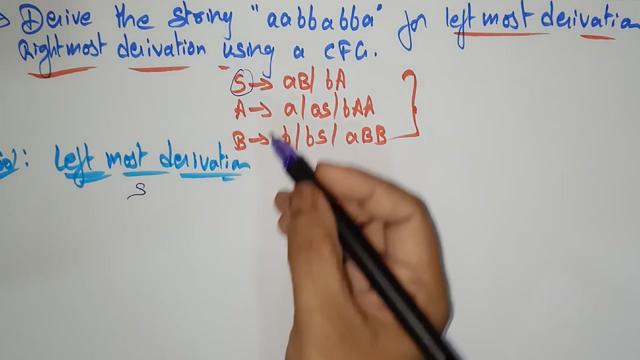 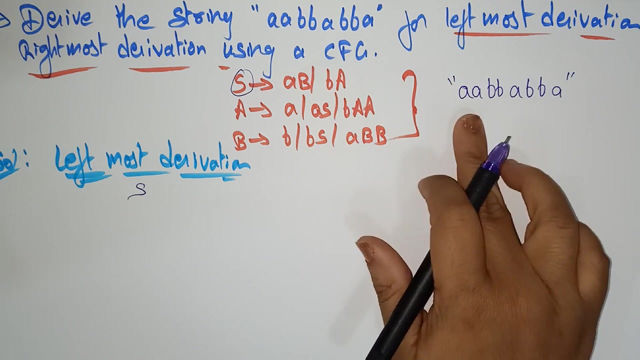 go with the leftmost derivation. Leftmost derivation. Okay so in the leftmost derivation, first let me take the pen, So first starts with the start symbol S. So this is a string. Let me write the string here again: a, a, b, b, a, b, b, a. So I want to derive the string. Okay, so first S should. 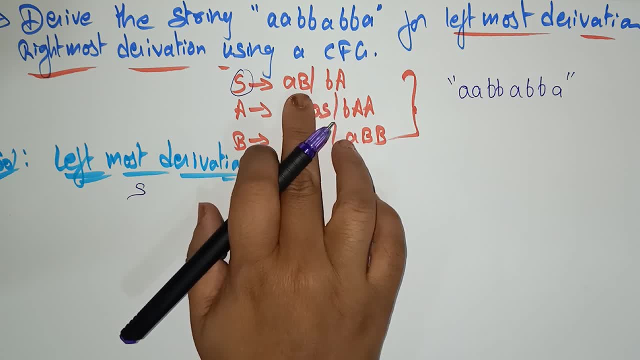 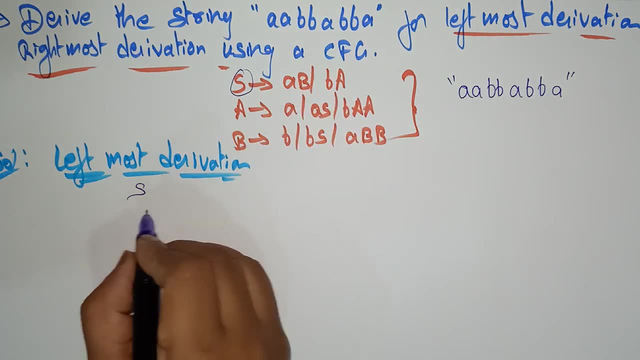 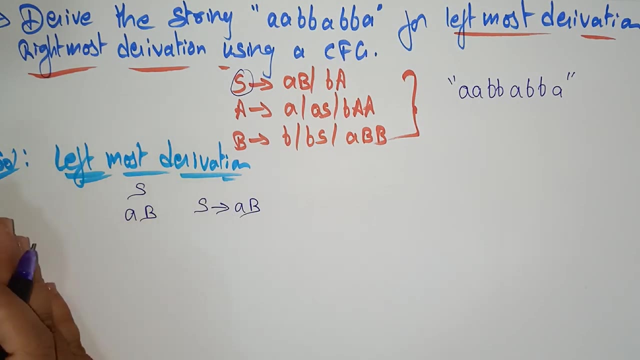 be. you have to take either a, b or b. Okay, so here the string will starts with the small terminal a, So I have to replace S as a b. Okay, S is replaced with a b. Now it's a leftmost derivation means you have. 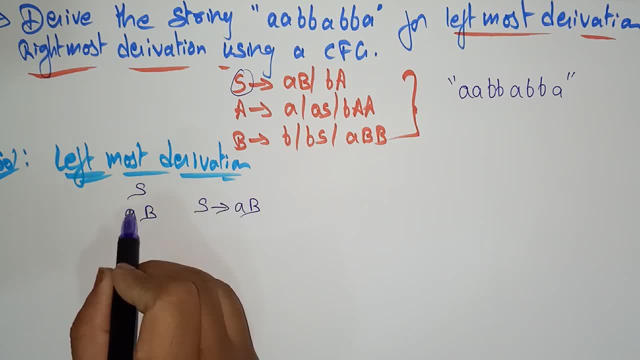 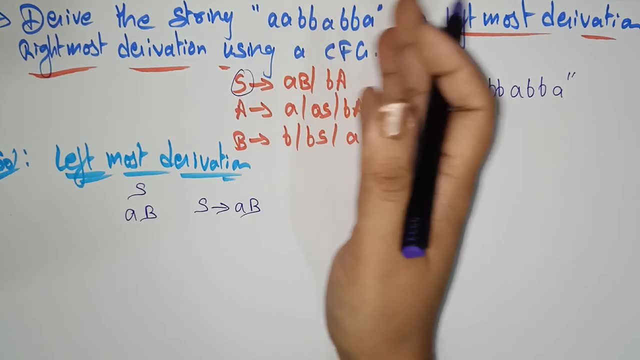 to start from the left left hand side. So, left hand side, This is a terminal, So you don't need to change. Now, coming to the non terminal, This non terminal should be replaced with the. this productions So a. So in the, in the place of b. 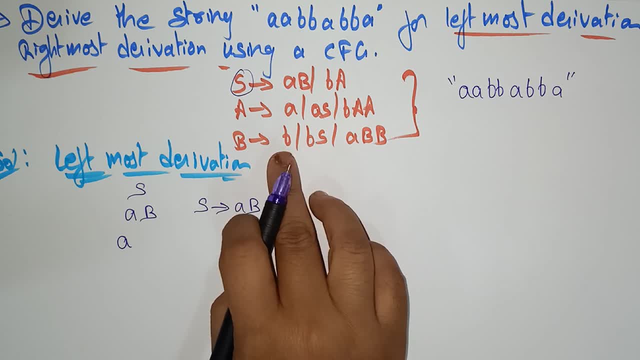 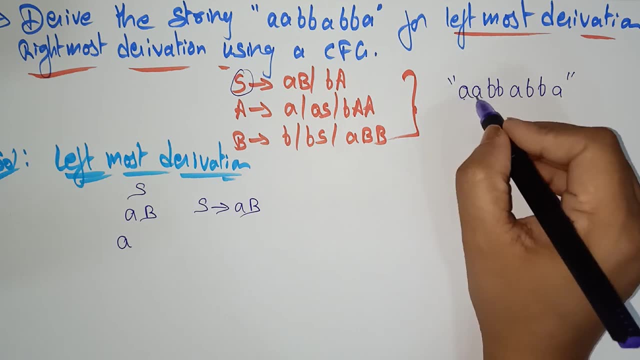 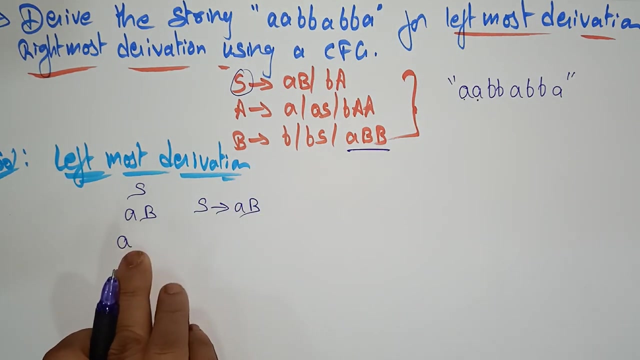 You have to replace the b with small b, bs or a b b. So according to our string, the next letter that comes from here in the string is sequence is a, So further you need to take a b b. So if you take, b means the string will be represented as a b, but it is not deriving our input string. If you take 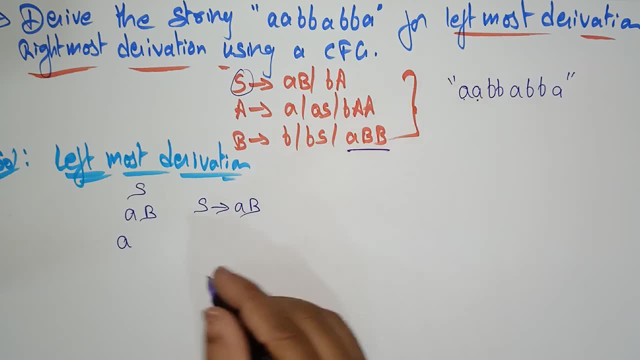 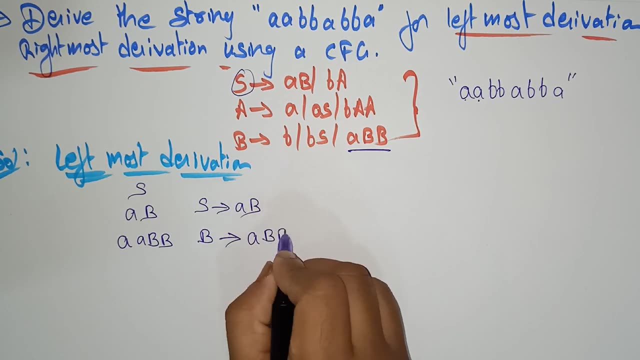 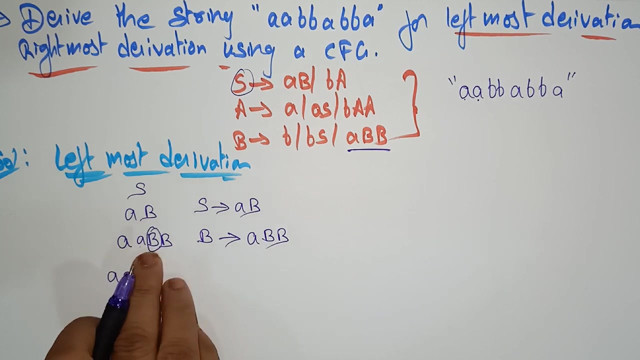 the bs. it is not deriving our input string, So I need to take a b, b, So the capital b letter that is replaced with a b, b. Okay, so this is a terminal and a is also a terminal. Now, coming to the first b. Okay, I have to take this b because this is a leftmost derivation, Leftmost. 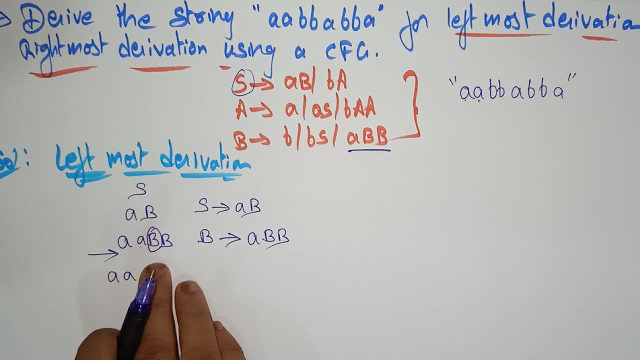 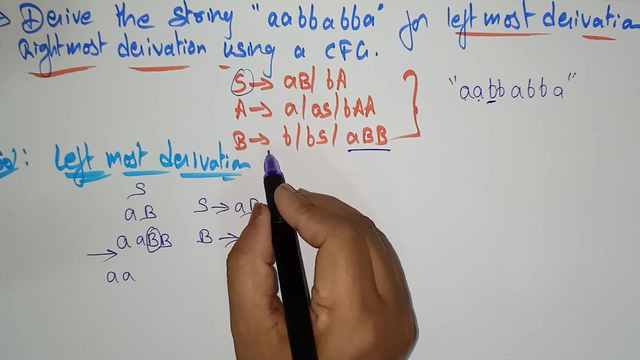 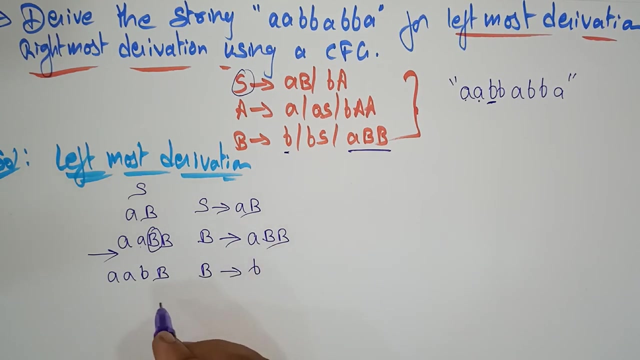 derivation means you have to take the first left non terminal that is present. So next is b. So in place of capital b, I need to replace with the small b, Small b, b. So b is replaced with the small b. Now a is a terminal, a is a terminal, b is a terminal. Now I have to replace this non terminal. 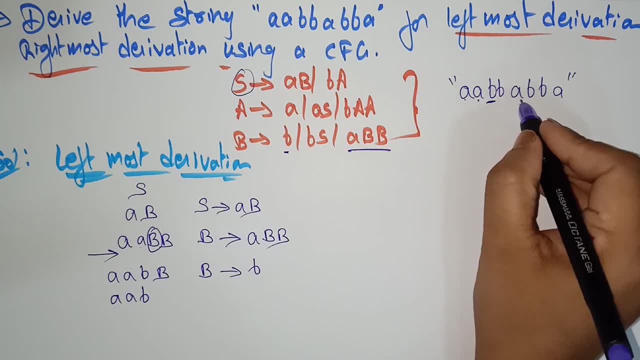 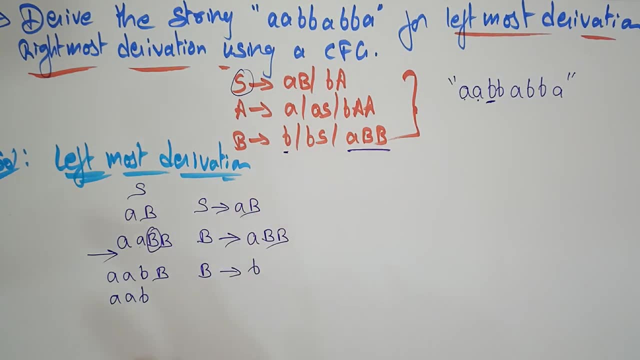 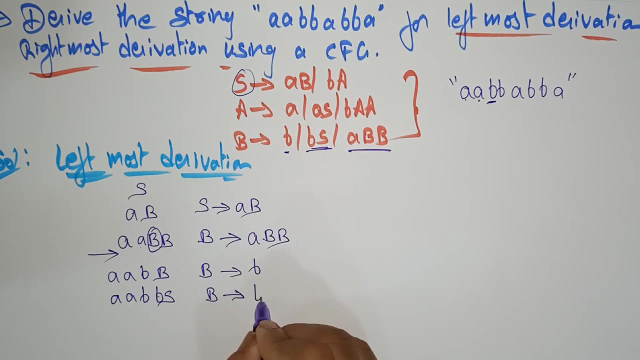 So with what letter? So here ba is there Next b? So if I replace with a, b, the string will end here, because there is no non terminals to replace. So I have to take bs. So bs I am taking. Okay, the b is replaced with the bs. Okay, so up to here the string is over. Now again a. 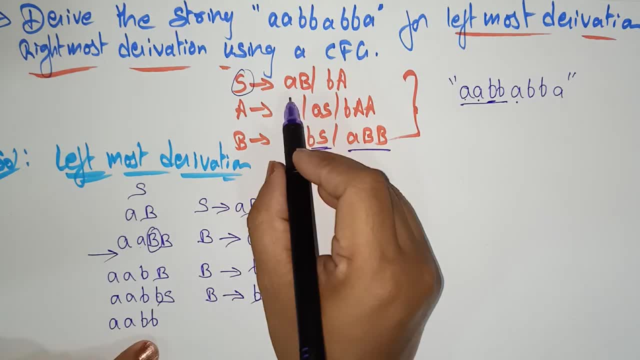 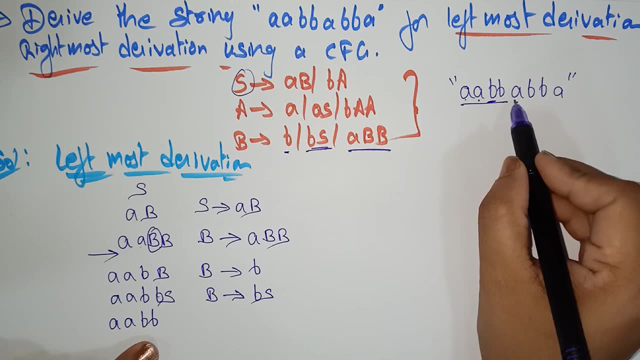 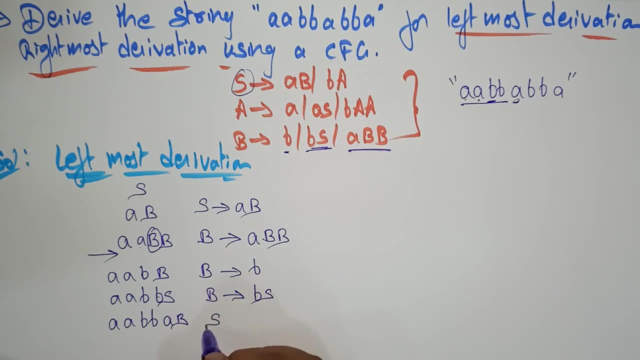 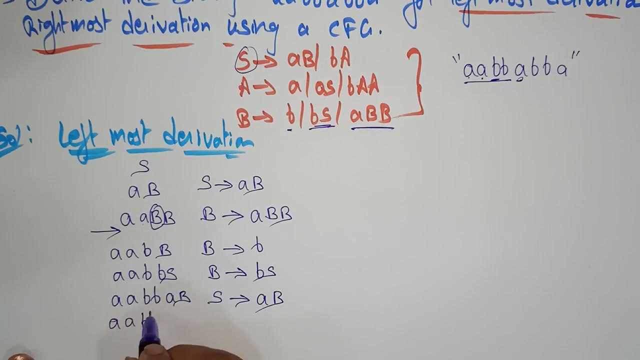 a, a, b, b is over. Now in place of s, what I have to take. Either I can replace s with a b or b a, But according to our derived string, the next after b, the a, is coming. So replaced s with a b. Okay, I replaced s with a b, Okay, so a is a terminal, a is a terminal b is. 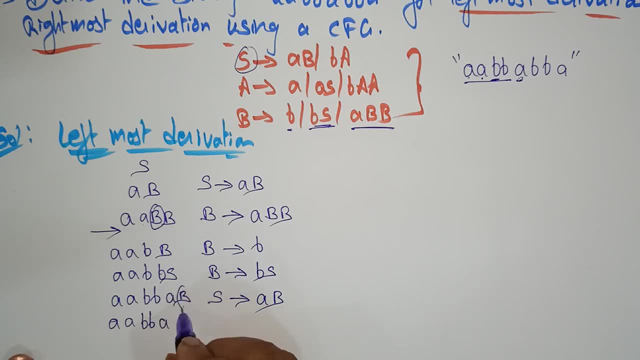 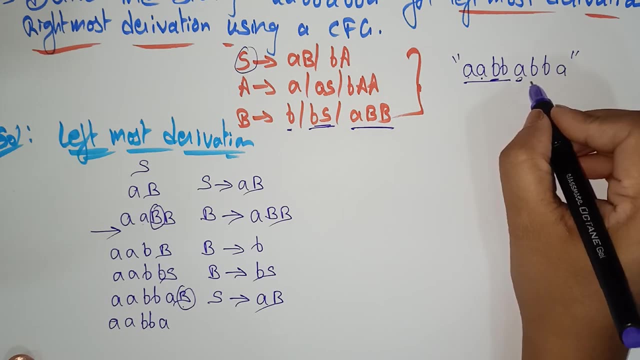 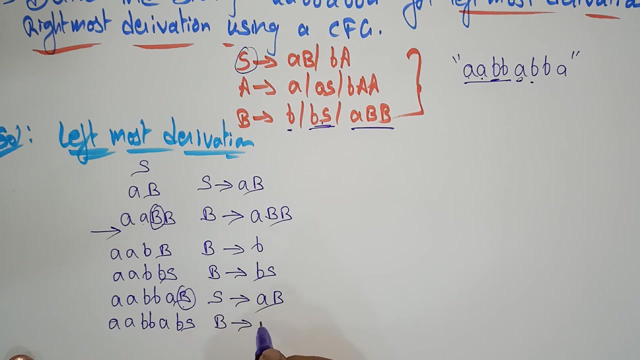 a terminal. b is a terminal and a is a terminal. Now, replace this b. I have to keep So the next. see the string, The next letter, that after a is a, b. So I want to replace this b with bs. Okay, b with bs. If you want, you can substitute b in place. 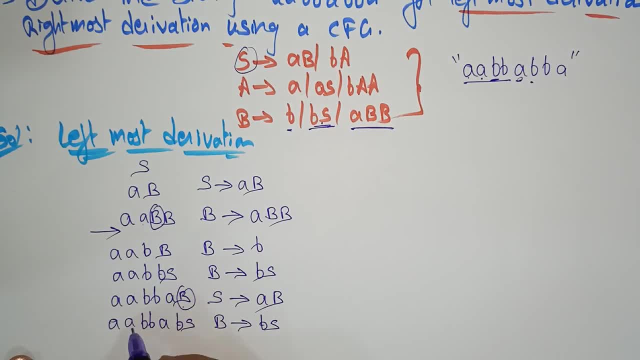 of b, you can write small b itself. Okay, then the string will end, But we have to derive this string. Okay, still, the remaining terms. here is the b. a is there. So I am replacing b with bs. Okay, so I have to keep. So the next see the string, The next letter that after a is a. 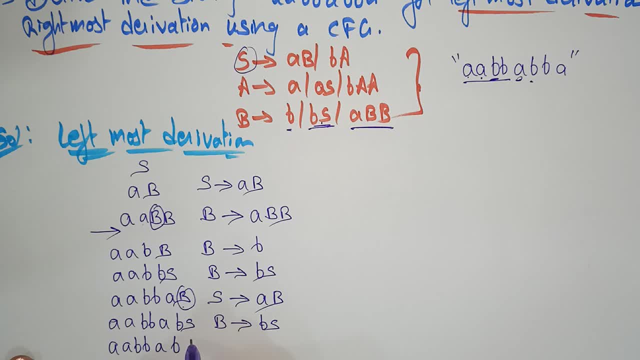 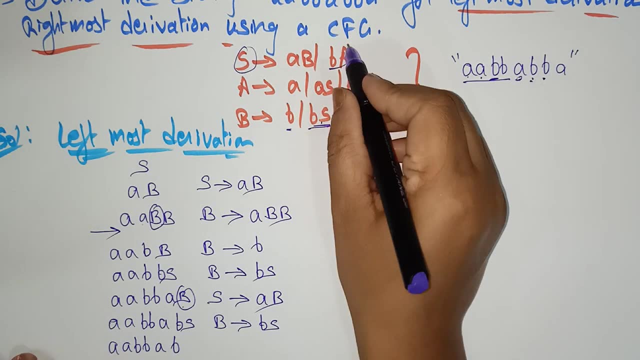 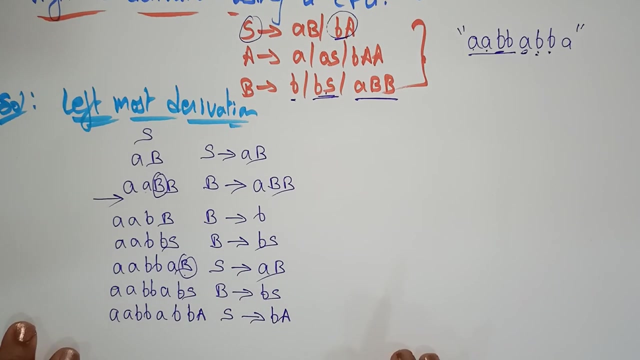 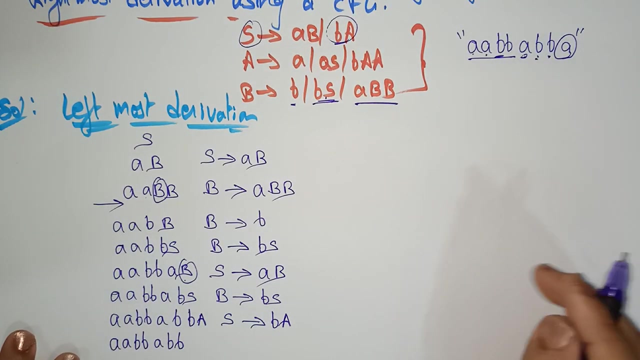 a, b, b, a, b. Now s coming to the s, What I have to take. So after a b, again b is there. So again b means I have to take this production. So s is replaced with ba, s is replaced with ba. So now a, a, b, b, a, b, b. escape The last. what is the last symbol in the string a? So 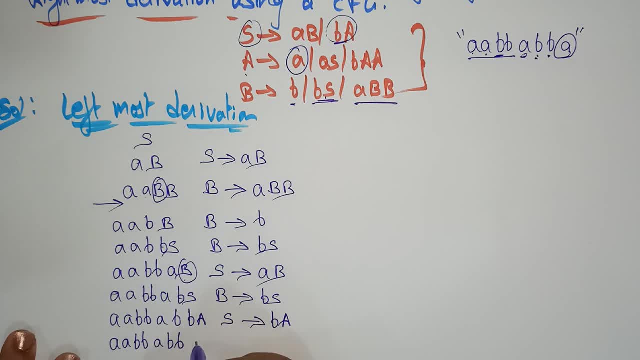 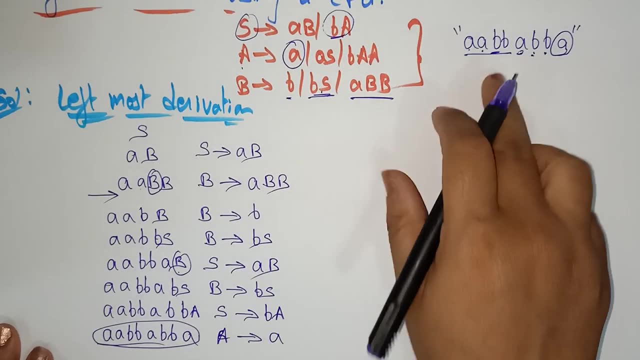 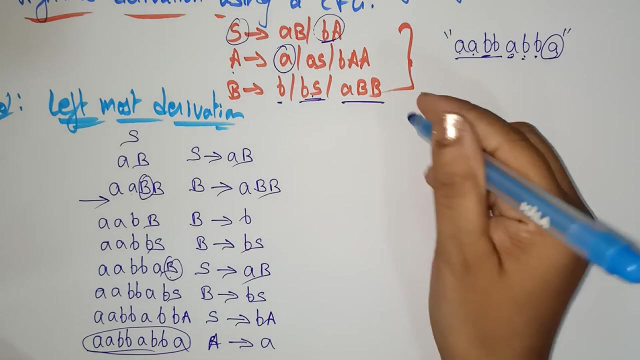 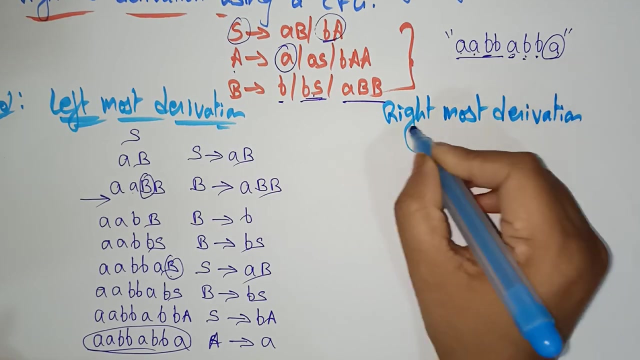 I have to replace a with a, So a capital a is replaced with the small a. So did I get the string derived? Yes, Whatever the input string they are. given that I derived by using the leftmost derivation, Now let me take the rightmost derivation this time. Rightmost derivation. Okay, So in the rightmost. 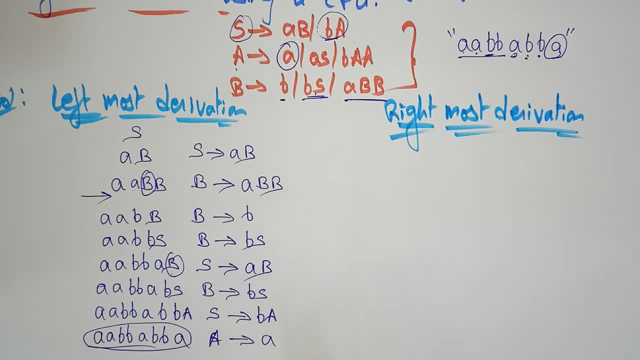 derivation I have to. a same procedure means the same in a string that you need to be derived, But you have to follow the procedure from right hand side. Okay, because this is the rightmost derivation. So s starts with a symbol, and this first what you have to take in place. 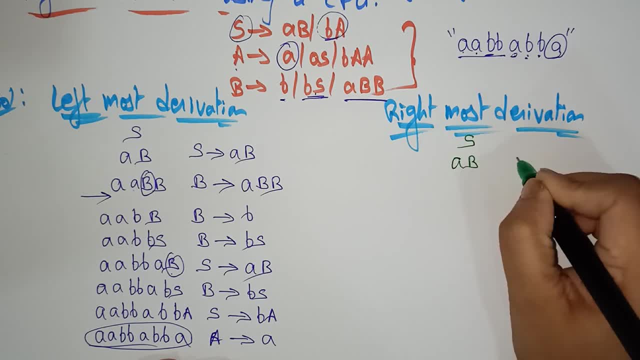 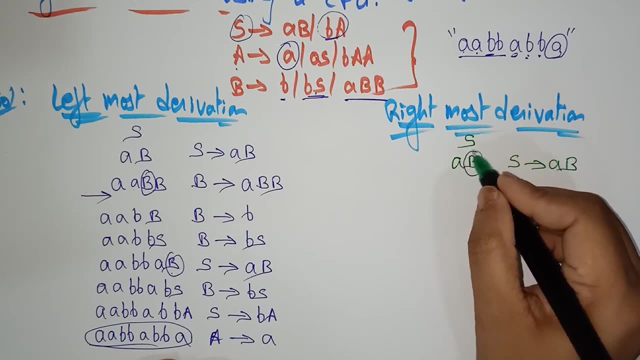 of s you have to replaced with a b. s is replaced with a, b. So now, the rightmost non-terminal, What is the rightmost non-terminal? b is the rightmost non-terminal, So replace b with a, b, b, Okay. 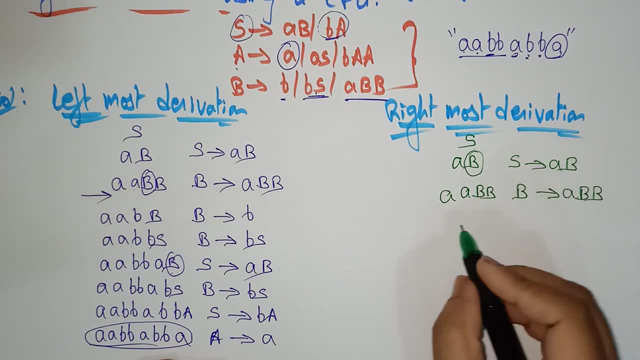 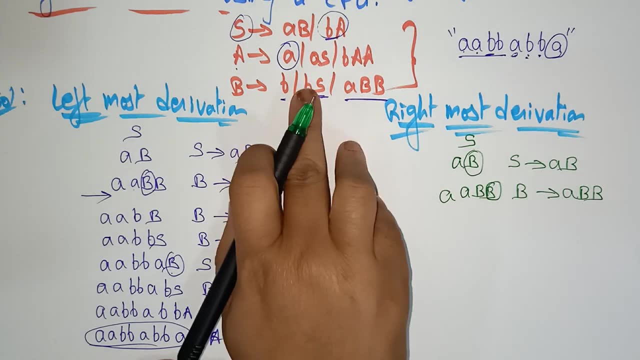 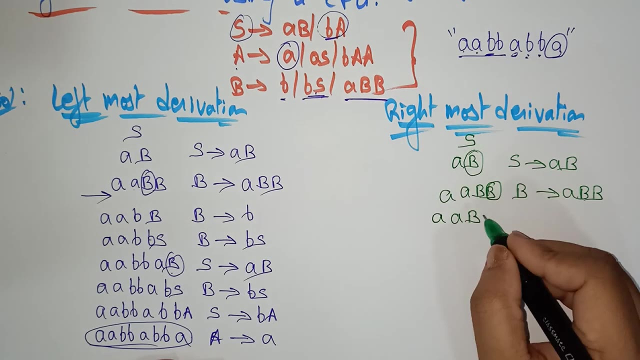 So replace b with a, b, b. So now, first, which terminal non-terminal I had to take, the rightmost non-terminal That has to be replaced with the productions. So a a, b, So last b. So what I had to take, I had to take b s in place of b. I am replacing with b is replaced with. 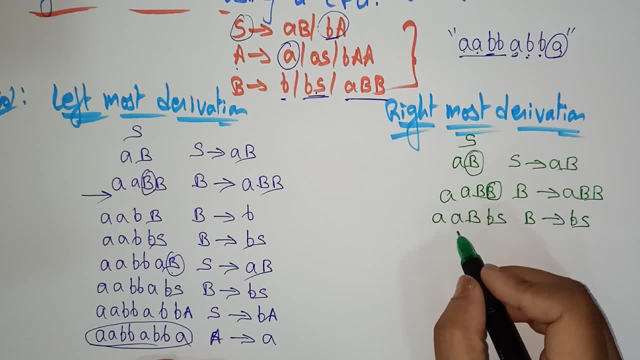 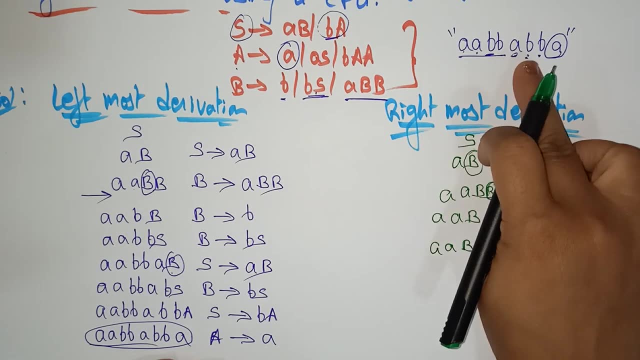 b, s. So in this string, what is the non-terminal? that is the rightmost, s is the rightmost, Okay, so a, a, b, b. so what is the last letter i have? i need to get? i need to get. it is a, so i'm replacing. 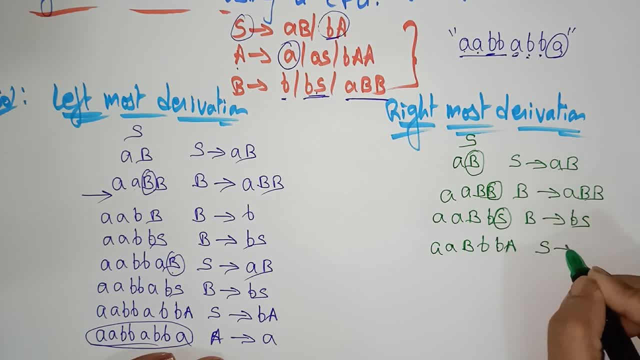 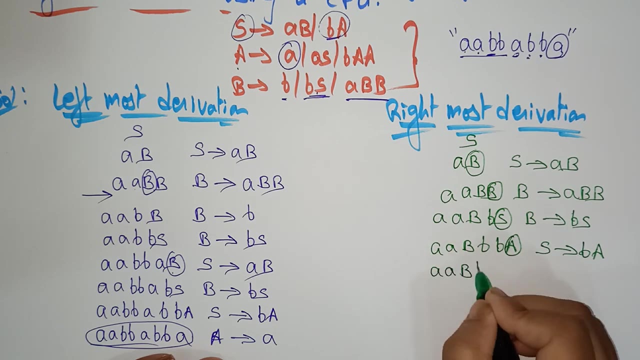 s with b a, so s is replaced with b a. and what is the last, rightmost, non-terminal a, so h, a i can replace with this small a, because b, b a string is forming, so a, a, b, b, a, so a is replaced with this small a. so up to here it is over. so this is. these are all the terminals, the right coming. 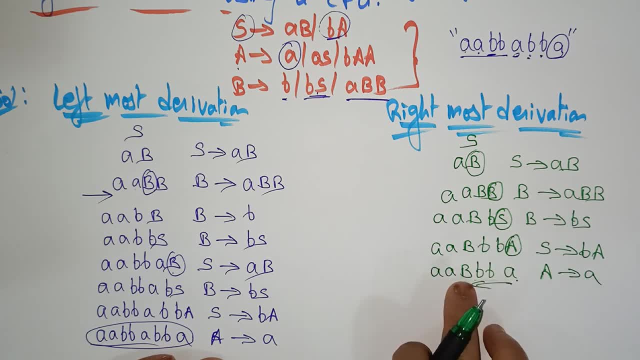 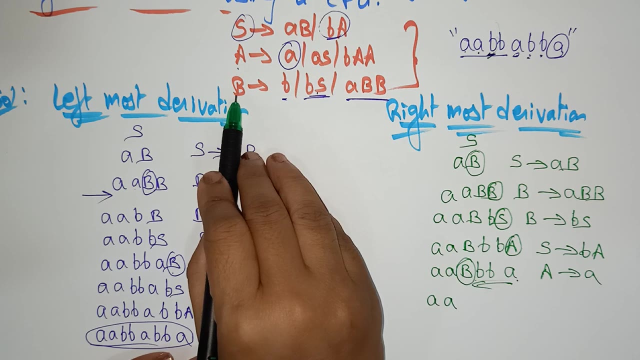 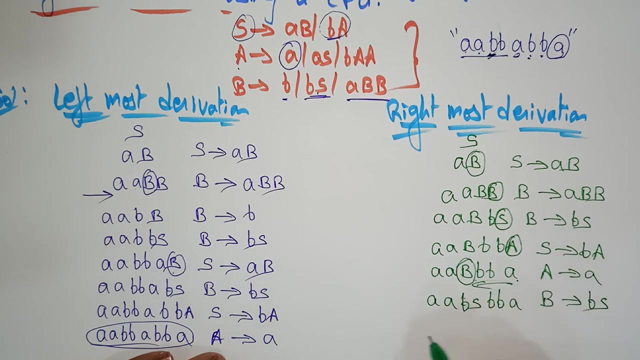 this way, because this is the rightmost derivation. okay, what is the next non-terminal that is present, b, so a? a in place of b. the next letter should be a. terminal should be b, so in place of capital b, i'm writing b? s, b, b, a. capital b should be replaced with b? s.